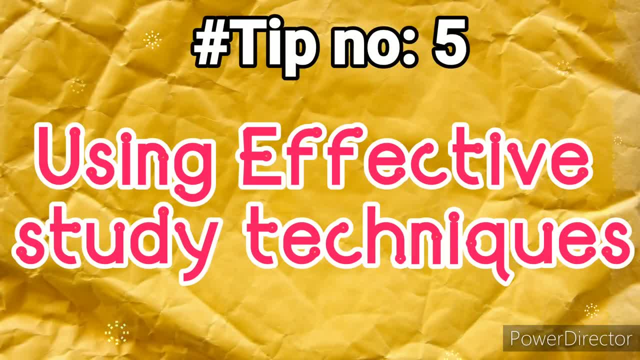 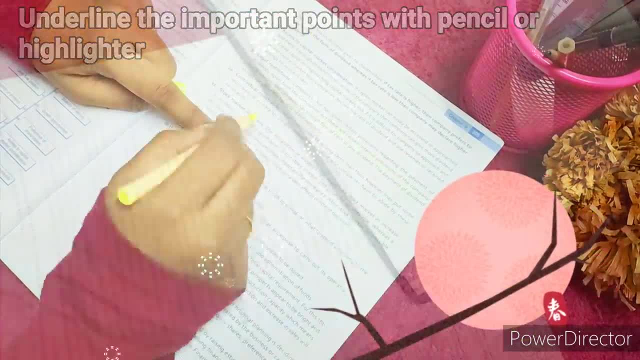 on each and every work. Tip number five: using effective study techniques. For, For example, when you start reading a chapter of any subject, just underline the points which you feel important. Make notes of your own by using some techniques, such as one-word questions, multiple choice. 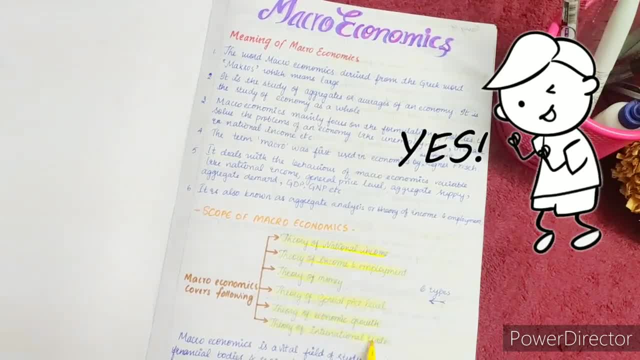 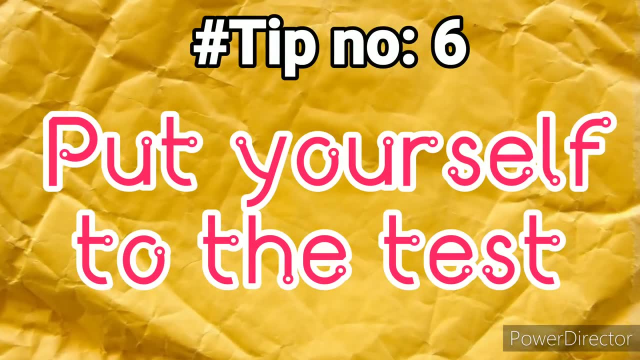 questions, diagrams, flowcharts, booklets, etc. This practice really helps you to score highest marks in your exams and it's 100% guaranteed Tip number 6. Put yourself to the test. Get into the routine of practicing question banks or question papers. 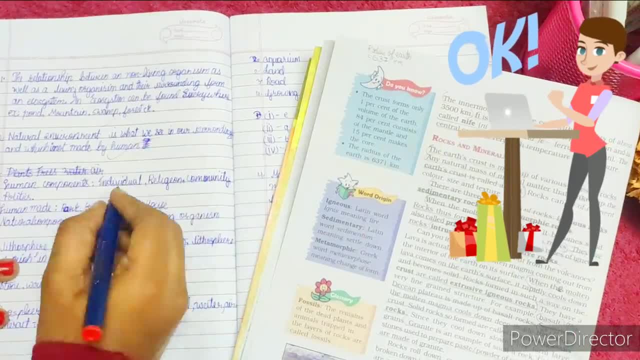 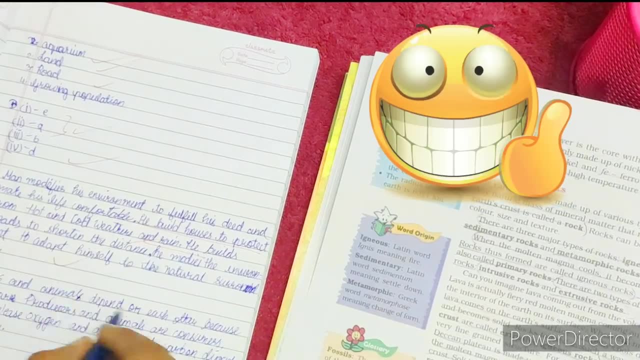 When you are done with a chapter, it's very important to take a small test paper on that particular topic which you have learnt. Now check the answers by yourself. This will really help you on what all mistakes you have gone through. This practice will give you lots of self-confidence. 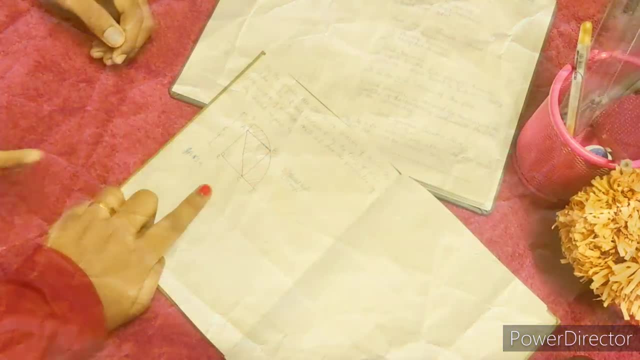 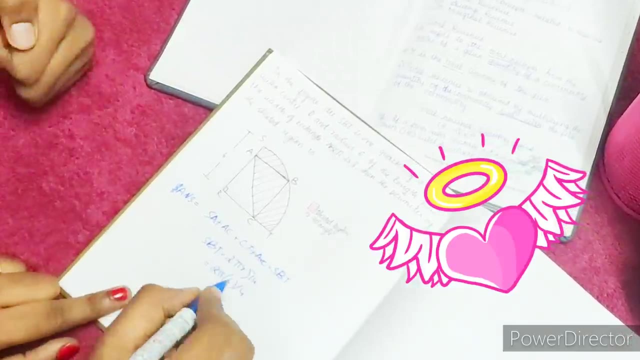 Tip number 7. Become a teacher. Explain your answers to others, especially to a friend who is not understanding that concept clearly. Help your friend by explaining it in your own words. This is probably the best way to learn when we teach them. 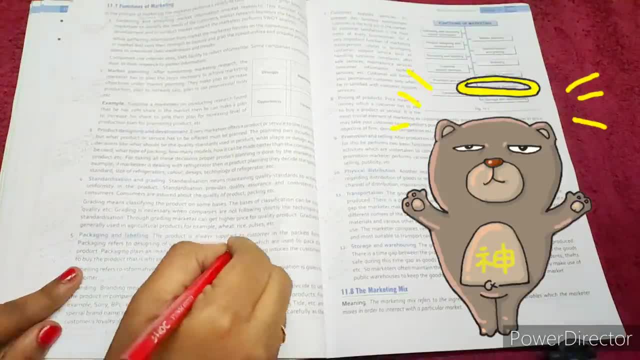 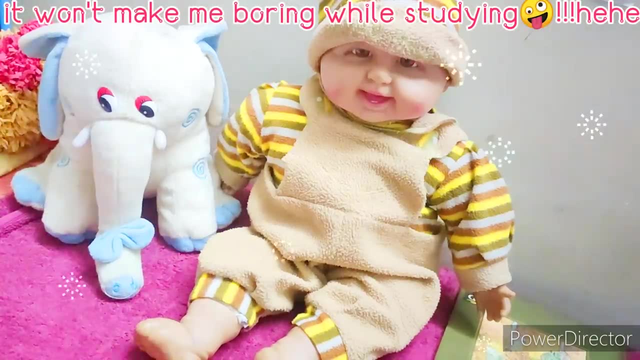 When I do my self-study, I usually imagine that I am a teacher and visualize my cute dolls and teddy bears as my students and I explain the answers to them on what topic I have learnt. This is also a very effective learning of self-study and gives you lots and lots of. 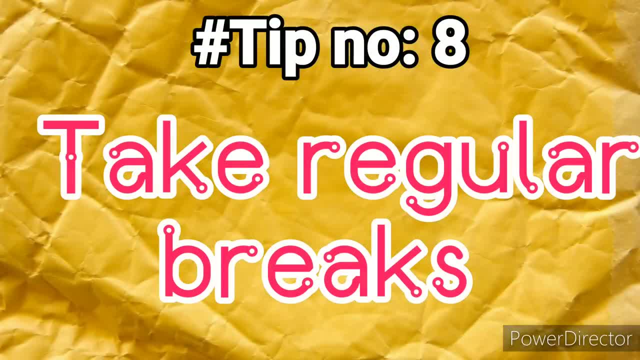 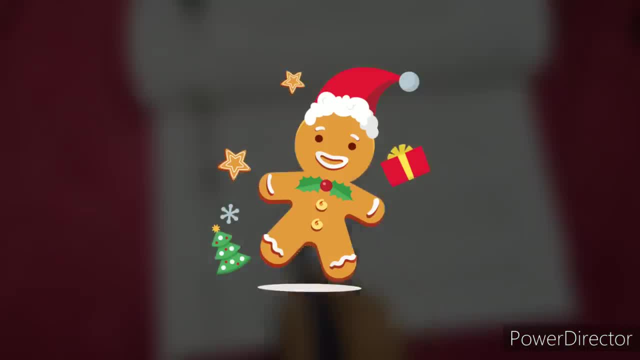 positive vibes and motivation. Tip number 8. Take regular breaks. If you are studying for a few hours at a time, take 5-minute breaks every half an hour or so. It helps your mind relax, which can help you more effectively remember the materials and 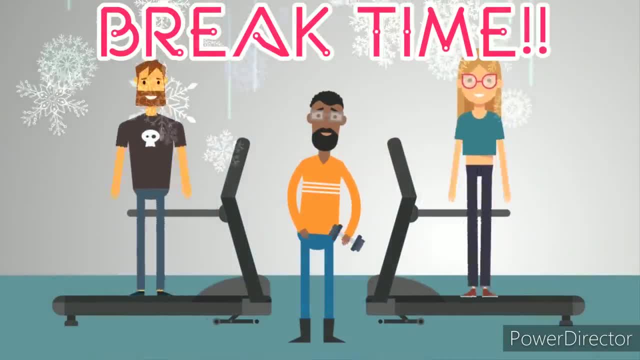 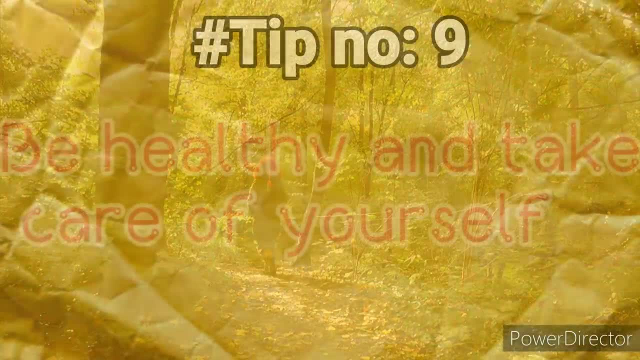 stay focused. In break time, you can do some physical activities, check out your social medias, read story books, watch television or just go for a walk. Tip number 9. Be healthy and take care of yourself. First of all, eat well. 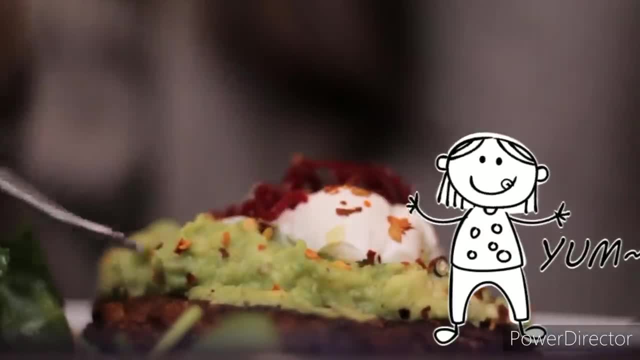 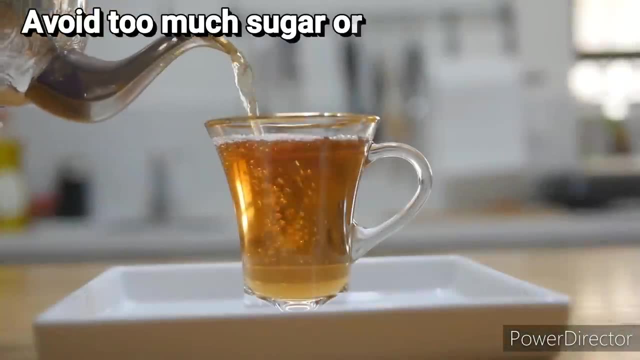 Food can help you to fuel your studies. Try this food to help your brain running at full power, such as protein rich food, fruits and vegetables, nuts and seeds. Avoid too much sugar or caffeine. that is, tea or coffee can interfere with concentration. Drink plenty of water.